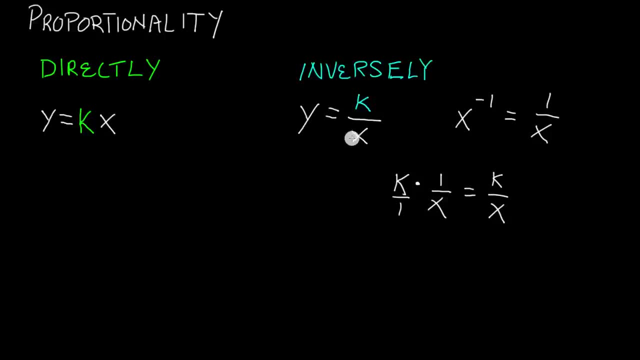 is a way that we can describe y being inversely proportional to x. So now that we've got that taken care of, let's go ahead and give our y's and x's and k's some values, so we can kind of illustrate what this really means with an example. Let's say that we were able. 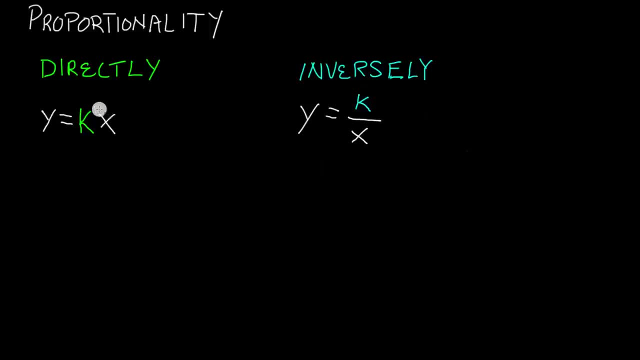 to measure both the variable y and the variable x and we found that at one time during the measurement y is equal to 6, and we found that x was equal to 3.. So we can kind of illustrate what this really means. So if we had a relationship between y and x, that was directly. 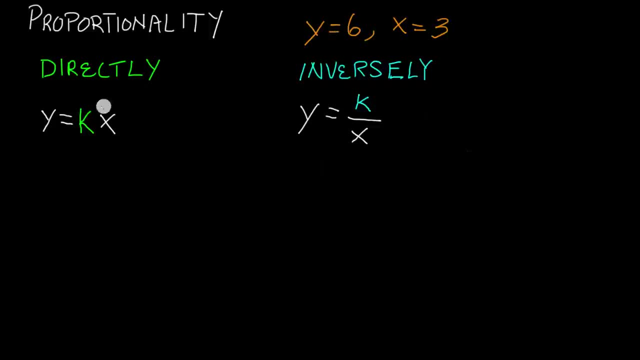 proportional, then we would simply plug in 6, where the y is here. 6 is equal to k, which we don't know what k is yet, but we know that x is equal to 3.. So at some time we were able to. 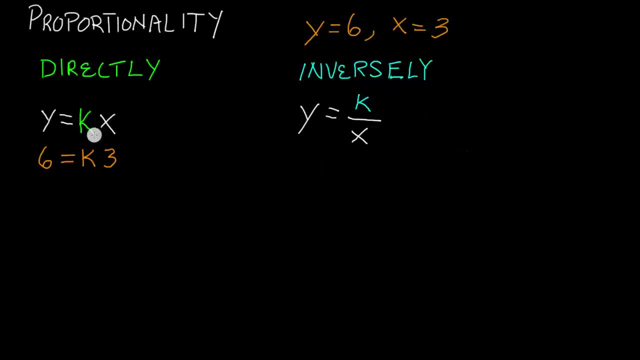 measure both y and x and in addition to that we know that y and x were directly proportional, then we would look at this relationship right here. 6 is equal to k times 3.. Well, we can divide the left and right-hand side by 3, so let's go ahead and do that. 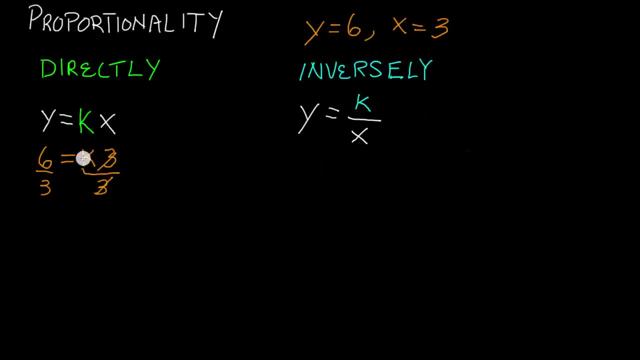 Divide the left and right-hand side by 3.. 3 over 3 cancels, leaving us with k on the right-hand side, And 6 divided by 3 is equal to 2.. If we were able to measure y equals 6 and x equals 3, and we knew that y was directly proportional to x, then that means that our 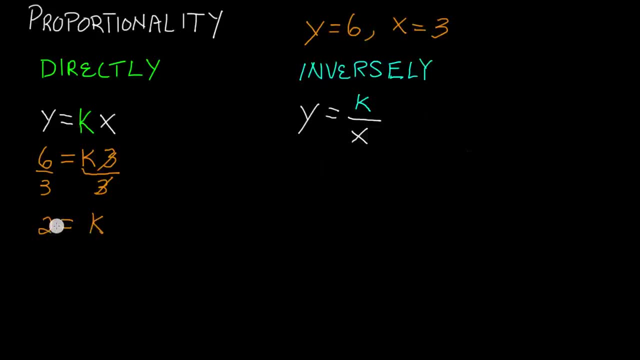 proportionality constant, k would be equal to 2.. So let's go ahead and put that together. Let's put that up here. Since we're using green for directly proportional, we'll just go ahead and write: k is equal to 2 in green. So 2 is our proportionality constant when. 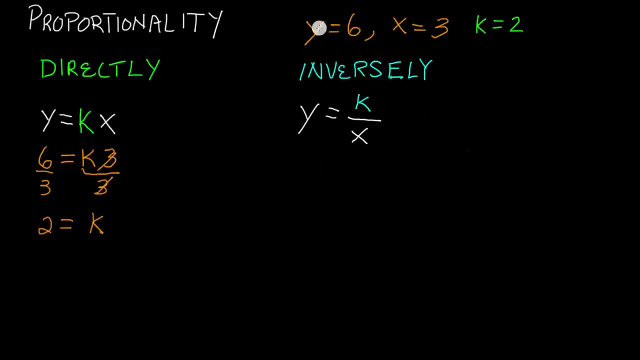 y is directly proportional to x, assuming that we were able to take the measurements: y equals 6 and x equals 3.. So now let's see what would happen if y was inversely proportional to x and we also measured the same values: y equals 6 and x equals 3.. 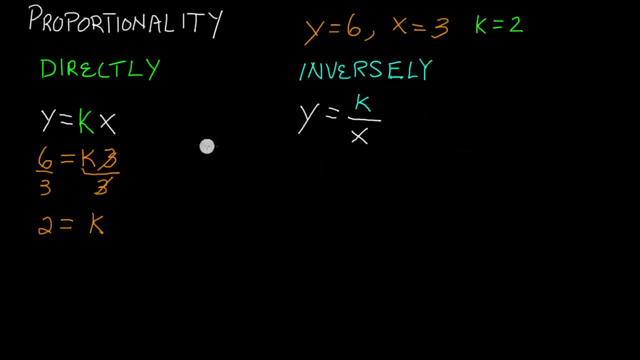 So in this case we just follow what we did In the directly proportional step. we say that y is equal to 6, right here. so we're just going to put a 6 where the y is, and that's equal to k divided by x And x. we said 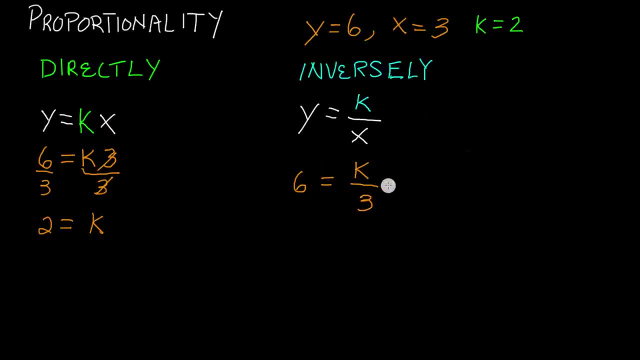 that we measured to be equal to 3.. So in this case, we would want to multiply the right-hand side and the left-hand side by the number 3.. 3 divided by 3 cancels, and then 3 times 6 is 18.. So right here we have. 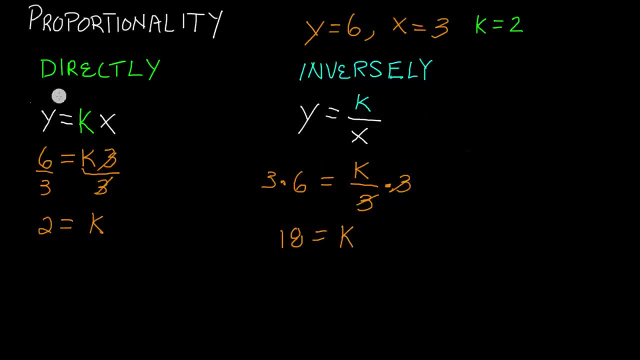 18.. Let's go ahead and write that in blue here now. So we have: k is equal to 18.. And I guess, maybe to make this a little more clear, I'll put ki here for inversely proportional, And then in the green I'll go ahead and put kd for the directly proportional. 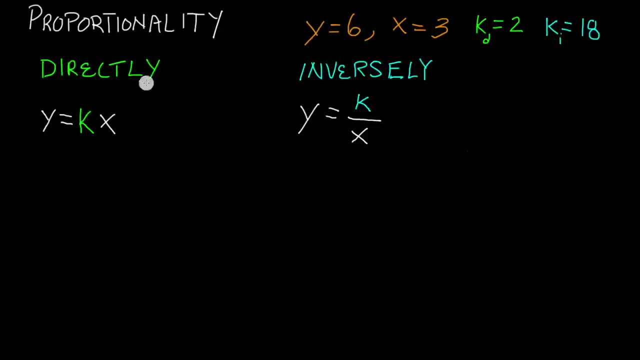 So, in a nutshell, what this means is that if we knew that we had a relationship where y was directly proportional to x And we were able to measure the values y equals 6 and x equals 3 at one instance during this relationship, Then we figured out that the proportionality constant has to be equal to 2.. 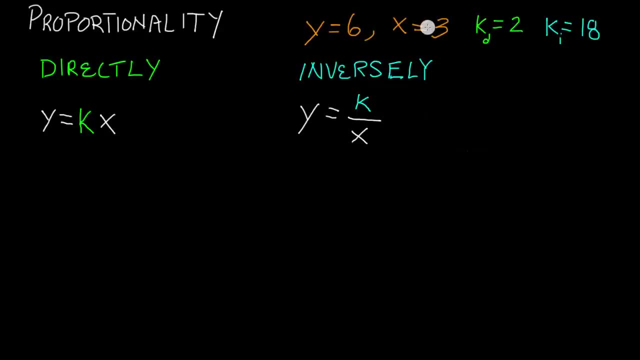 On the other hand, if we had those same two measurements and we knew that the relationship between y and x was inversely proportional, then we find out that our proportionality constant is actually equal to 18.. So now let's take a look at what happens when we vary. 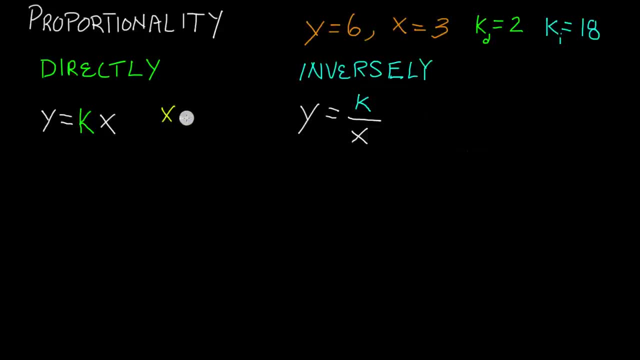 We'll just say that x is equal to 2.. So in both of these situations we know the proportionality constant in each of these cases. And so if y was directly proportional to x and we wanted to know what y was when x equals, 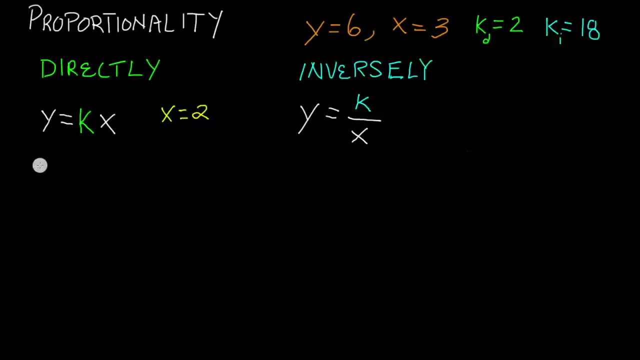 2, then we would just simply solve this problem right here. y is equal to. in the case that y is directly proportional to x, kd is equal to 2.. So we'll just go ahead and write 2, and then multiply that by our x, which we're just taking. 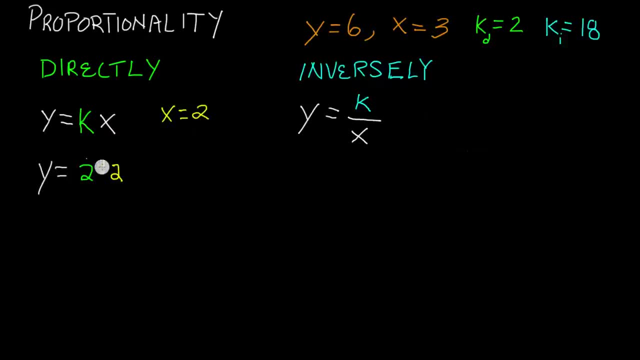 to be 2.. We want to know what y is when x is 2, and y is directly proportional to x. So if that was the case, then y is equal to 2 times 2, or y is equal to 4 when x equals. 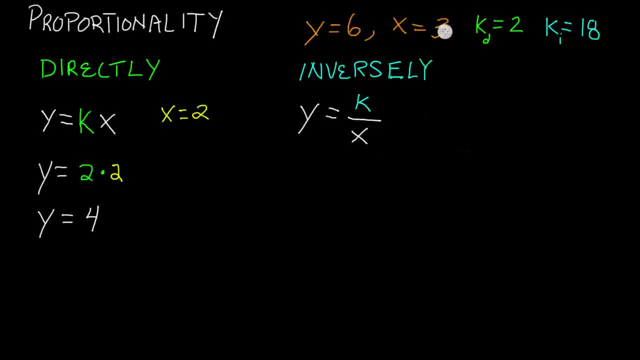 2.. On the other hand, if we measured that y equals 6 and x equals 3 in some instance of time and we also knew that y was inversely proportional to x, then we would use this proportionality constant here. and if we wanted to check what value y was when x equals 2,. 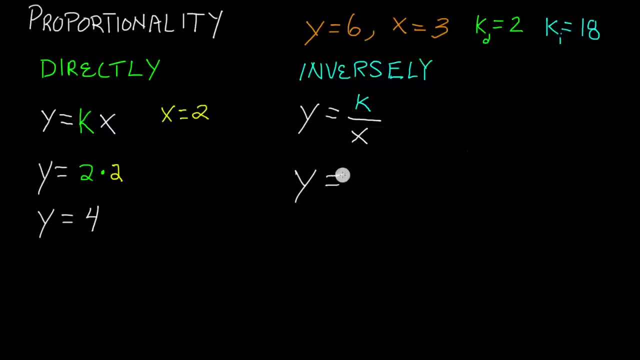 we would simply write: y is equal to, and this time we would write the proportionality constant where y is inversely proportional to x, and that would be 18.. That's 18 divided by, and then x, we're saying, is 2.. 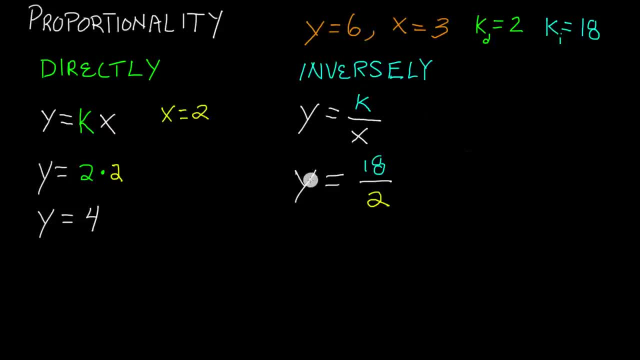 So we want to know what y will be when x is equal to 2, assuming that y has an inversely proportional relationship to x and that these were the measured values right here. So 18 divided by 2 is equal to 9.. 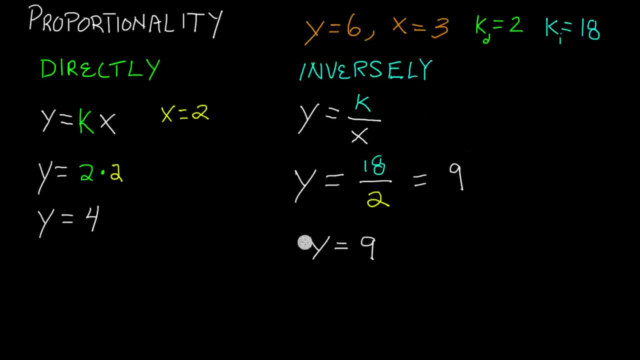 So for this case we got y is equal to 9.. And for the other case we got y is equal to 4.. So just to explain this one more time: on the left-hand side we have the relationship where y is directly proportional to x. 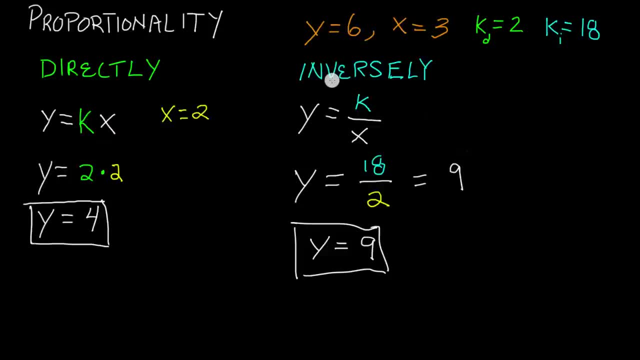 and k is our proportionality constant. on the right-hand side here we have a relationship where y is inversely proportional to x and k is also our proportionality constant. So we're kind of looking at these two cases separately and we're just assuming that we were able to measure. 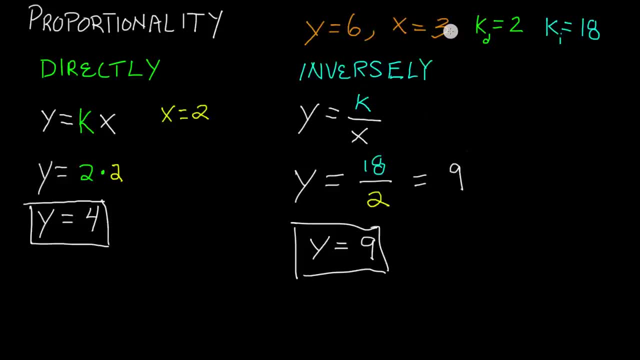 y equals 6 and x equals 3 at one moment in time when we were running some sort of experiment where we're measuring y and x. So if y was directly proportional to x, then we would determine that our proportionality constant is 2.. 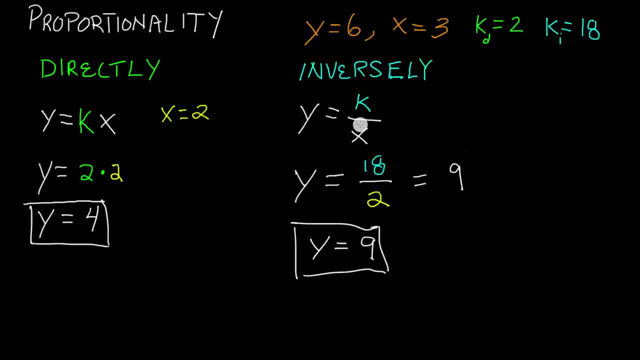 On the other hand, if y was inversely proportional to x and we measured that y equals 6 and x equals 3, then we would determine that our proportionality constant is equal to 18.. So in both of these cases, we're then checking to see. 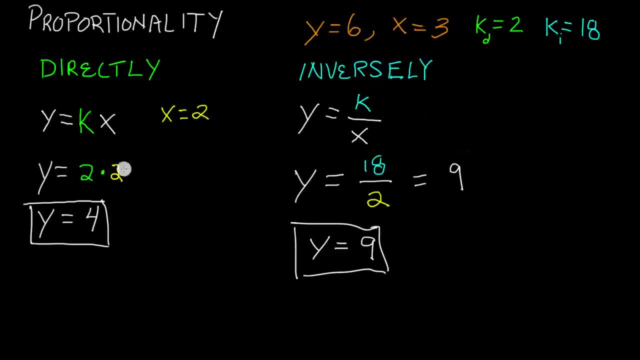 what the value of y would be if x was equal to the value 2. based on the previous conditions For the directly proportional case, where we're using the proportionality constant of 2, we find that y is equal to k times x or 2 times 2,. 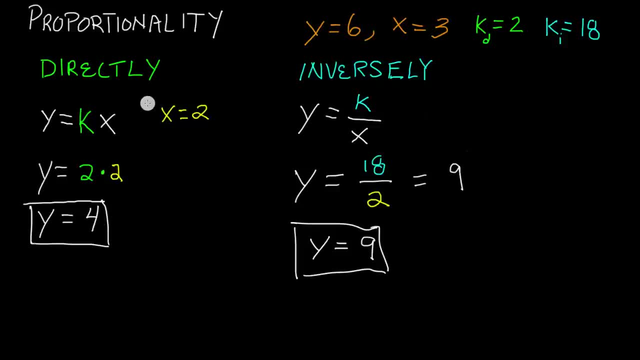 and y would be equal to 2.. y is equal to 4 in the directly proportional case. On the other hand, in the inversely proportional case we would have: y is equal to k divided by x, and this time we're using the proportionality constant. 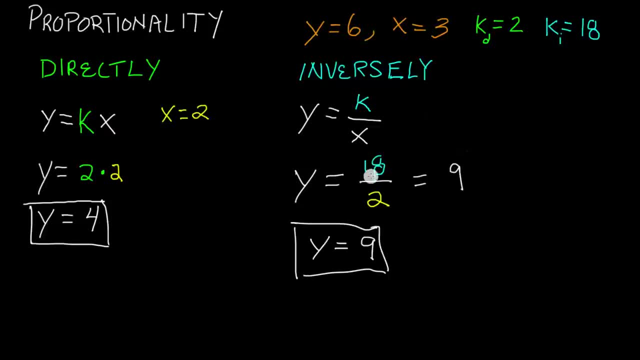 for the inversely proportional relationship. So we have 18 divided by 2, which is equal to 9.. So I hope that makes sense to you guys who are trying to understand proportionality. The two main kinds of proportionality are directly proportional and inversely proportional.